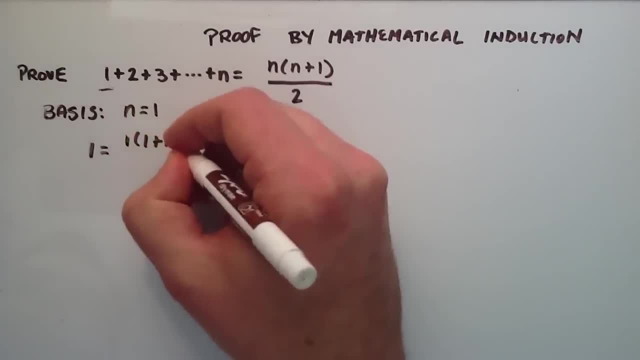 So this becomes 1 times 1 plus 1 divided by 2.. And then we just are simply checking to see if the right hand side is equal to the left hand side. for this base case, 1 plus 1 is 2.. We multiply that by the 1 on the left here. 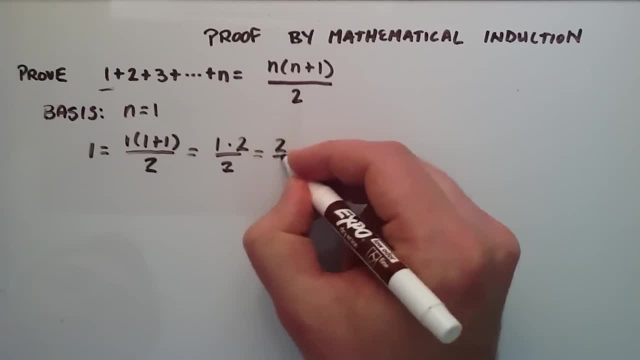 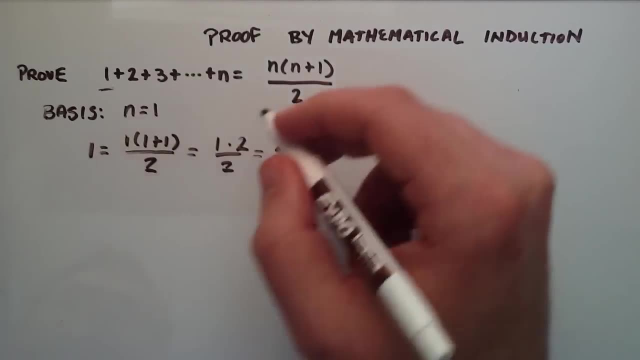 Divide that by the 2 on the bottom, 1 times 2 is 2. divided by the 2 on the bottom is simply equal to 1.. So for the base case for n equals 1, we have basically: 1 on the left hand side equals 1 on the right. 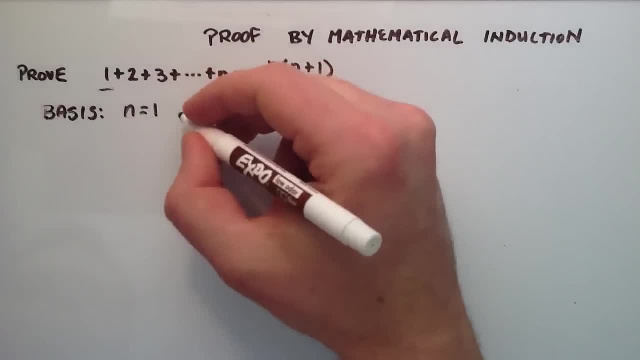 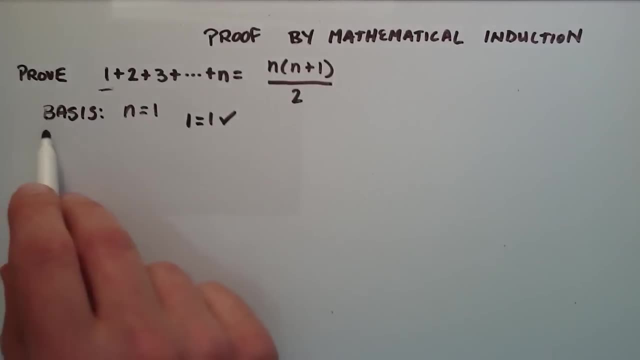 And then we just write down the value 1 on the left hand side. So I think that's simple enough. We can just erase it. So basically, for the base case we have: 1 equals 1, and that is a true statement. 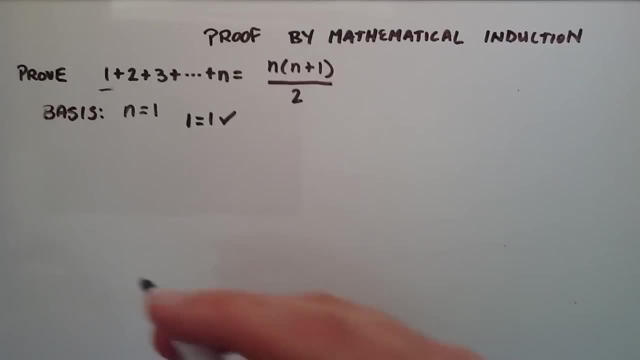 And so, since the base case is true, we can proceed to the next step. So the next step is going to be the induction step And basically what we're going to do with the induction step is we're going to do a couple things. 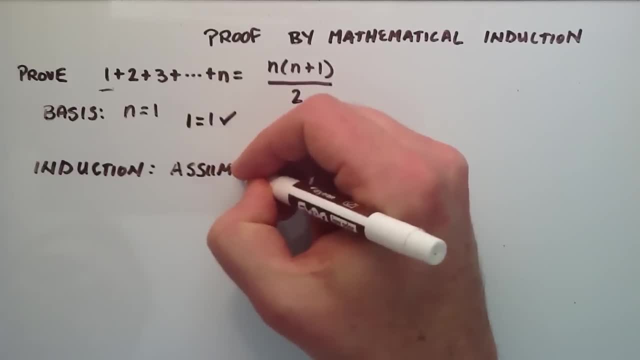 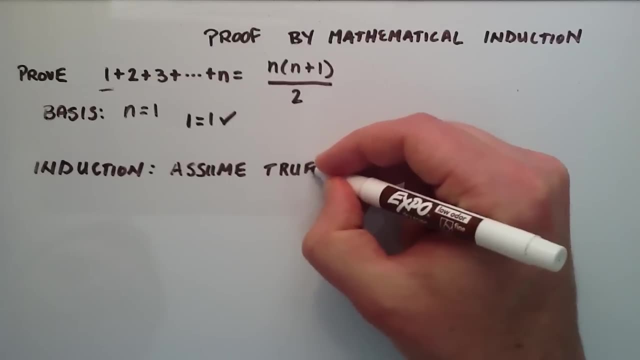 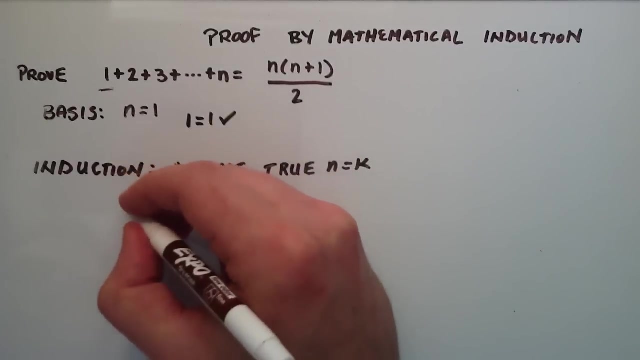 We're basically just going to assume, Assume, Assume- that this statement is true for some value: n equals k. So we're going to assume that it's true for n equals k, And so basically, let's go ahead and do that now. Let's just say that we have 1 plus. 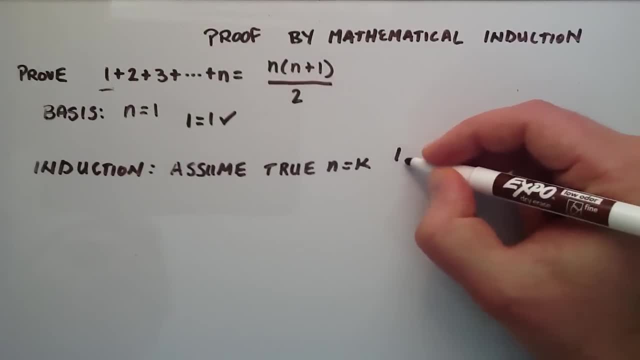 Let's write it over here to give myself some more room. So basically, for this step we have 1 plus 2 plus 3 plus all the way up to some value k. We're saying that we're just going to do the induction step. 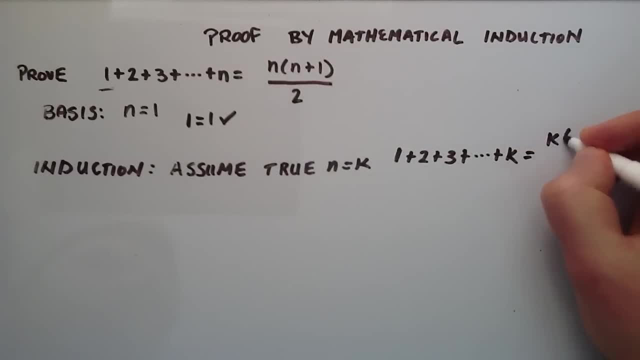 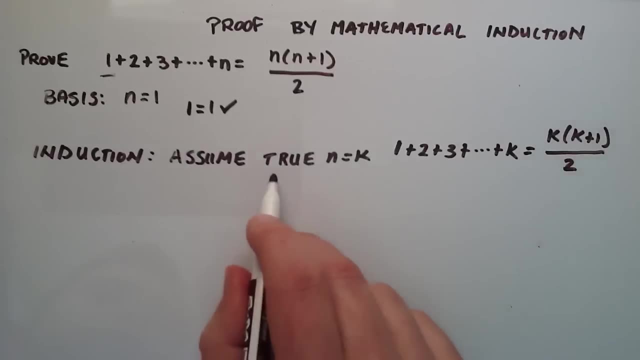 It's just going to assume that that's equal to the right-hand side, So plugging in k, where n's are k plus 1 divided by 2.. So we've assumed that this is true, And so then the next thing we want to do is we want to show that it is true, for n is equal. 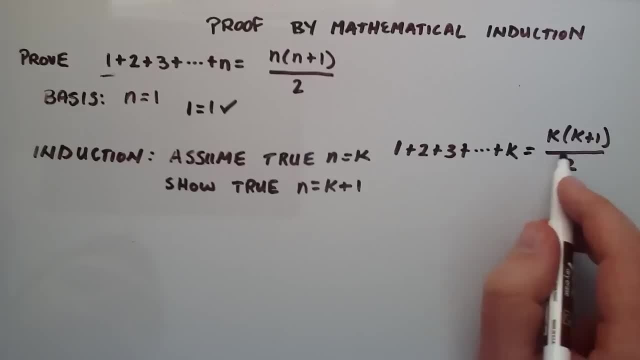 to k plus 1.. So we've assumed this step is true. for n equals k. We're going to show that it's true for n equals k plus 1.. plus one, and we're going to do that based off of this assumption. So for n equals k. 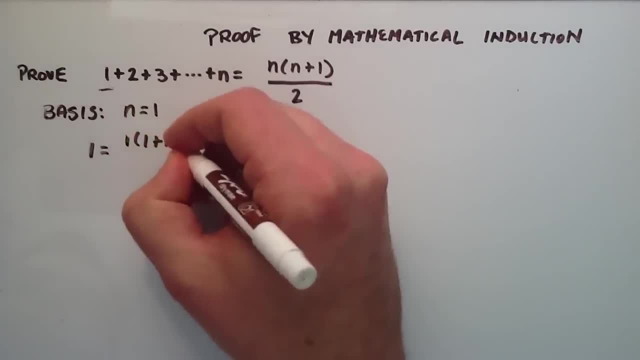 So this becomes 1 times 1 plus 1 divided by 2.. And then we just are simply checking to see if the right hand side is equal to the left hand side. for this base case, 1 plus 1 is 2.. We multiply that by the 1 on the left here. 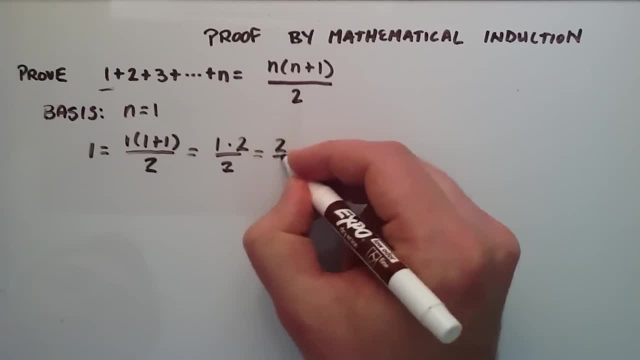 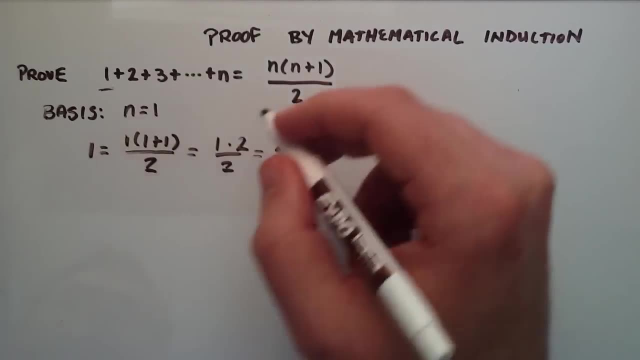 Divide that by the 2 on the bottom, 1 times 2 is 2. divided by the 2 on the bottom is simply equal to 1.. So for the base case for n equals 1, we have basically: 1 on the left hand side equals 1 on the right. 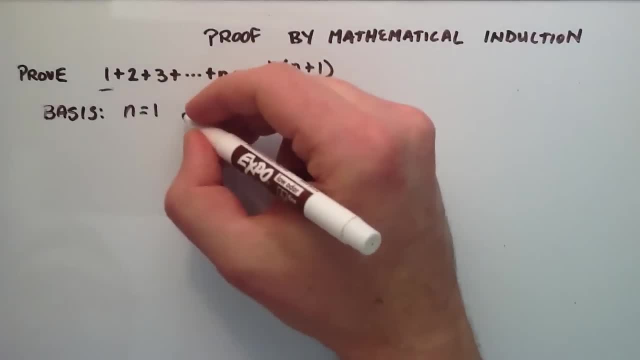 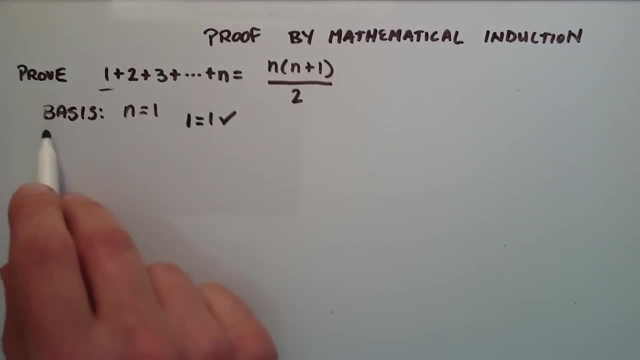 And then we just have the left hand side. So I think that's simple enough. We can just erase it. So, basically, for the base case, we have: 1 equals 1 and that is a true statement. And so, since the base case is true, we can proceed to the next step. 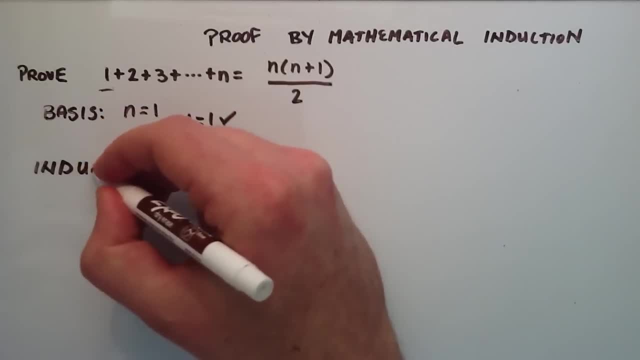 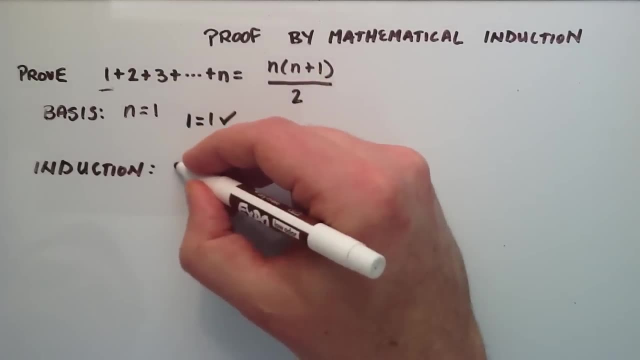 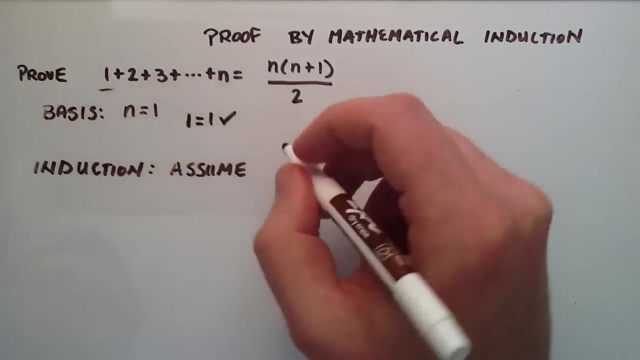 So the next step is going to be the induction step And basically what we're going to do with the induction step is we're going to do a couple things. We're basically just going to assume, Assume that this statement is true for some value. n equals k. 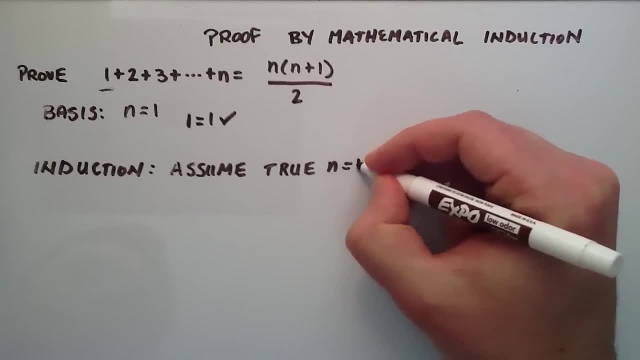 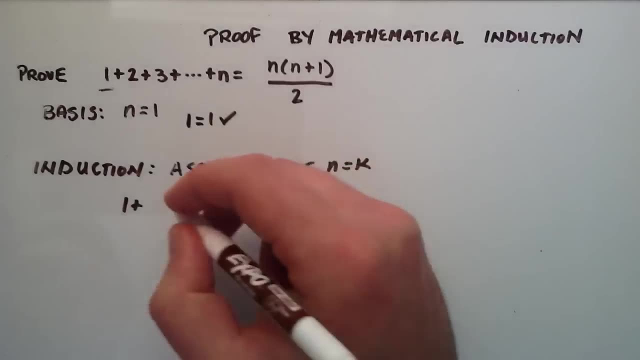 So we're going to assume that it's true for n equals k, And so basically, let's go ahead and do that now. Let's just say that we have 1 plus. Let's write it over here to give myself some more room. 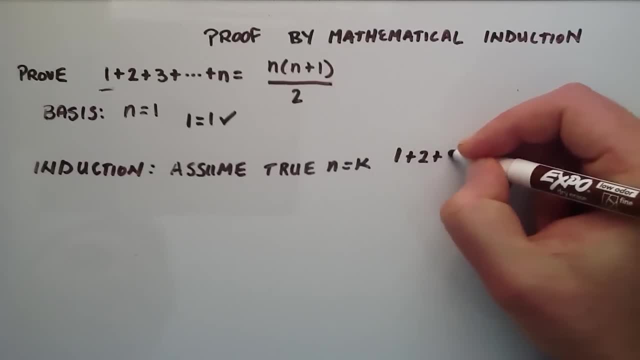 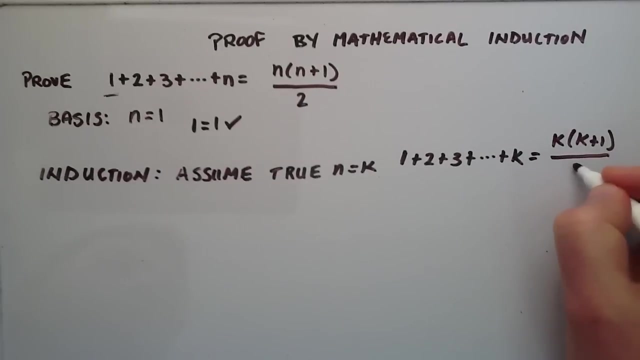 So basically for this step we have 1 plus 2 plus 3 plus all the way up to some value, k. Okay, So we're just going to assume that that's equal to the right hand side, So plugging in k where n's are k plus 1 divided by 2.. 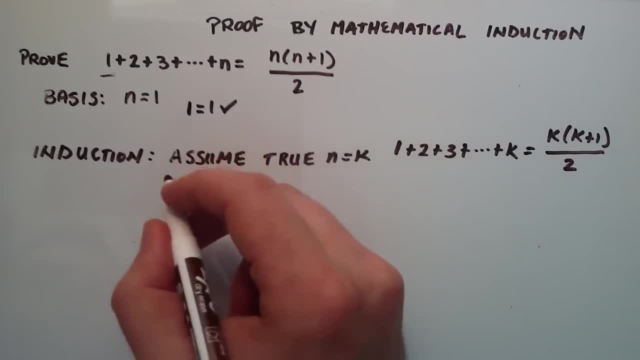 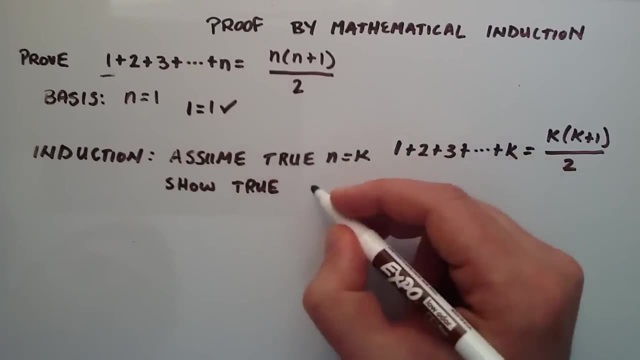 So we've assumed that this is true, And so then the next thing we want to do is we want to show that it is true, for n is equal to k plus 1.. So we've assumed this step is true: for n equals k. 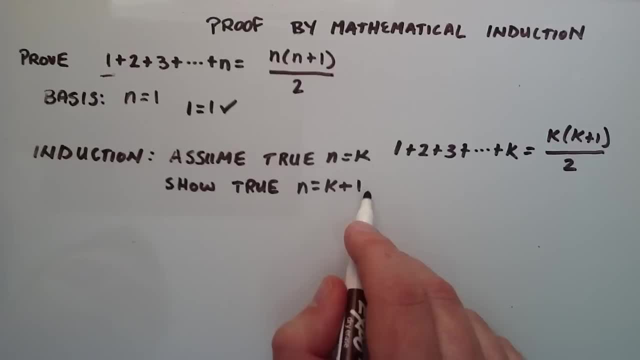 We're going to show that it's true: for n equals k plus 1.. And we're going to do that based off of this assumption. So for n equals k plus 1, we basically have 1 plus 2 plus 3, plus all the way up to k. 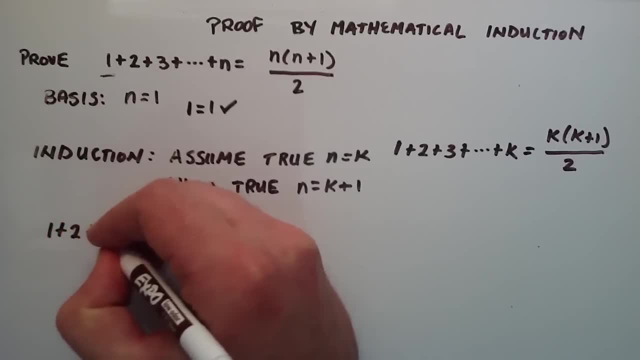 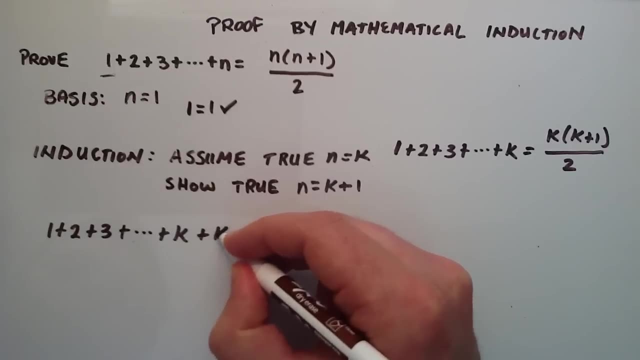 plus one. we basically have one plus two plus three, plus all the way up to k, and then we go one more further to k plus one, and then we're going to also plug in k plus one where the n's are here. So this is going to be k plus one for that part, and that's multiplied. 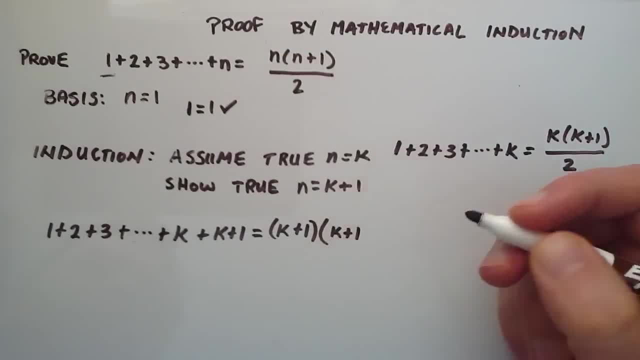 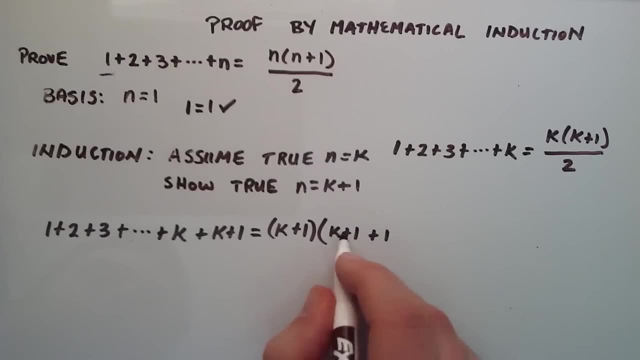 by k plus one, plugging that in where the n is, and then we have a plus one. We could put this in parentheses to kind of set it apart, but really we're just going to be adding these anyway, so I'm just going to leave it like this, And then we're going to divide that. 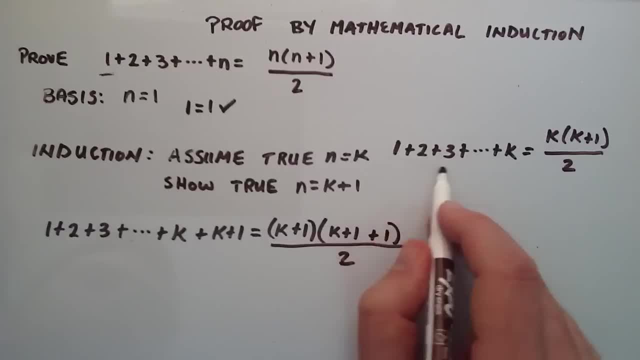 by the two here. So we're assuming this is true and we're going to show that this is true based off of this assumption. So what we're going to do with this assumption is, if you notice, right here we have one all the way up to k. so that's the same as what we have right here. And since we're assuming- 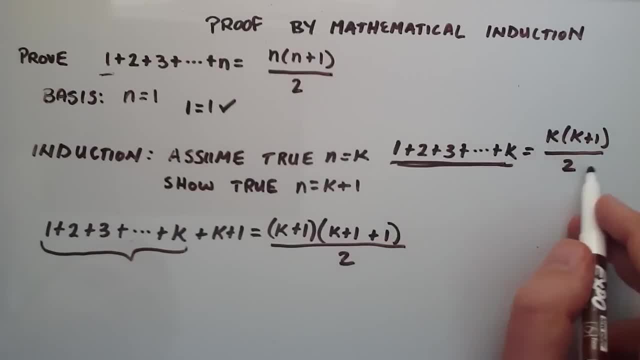 this is true, then we're basically saying that this right here we can use to replace this, because these are the same. So we're just going to replace all this stuff with the right hand side of this assumption. So this becomes k times k plus one. 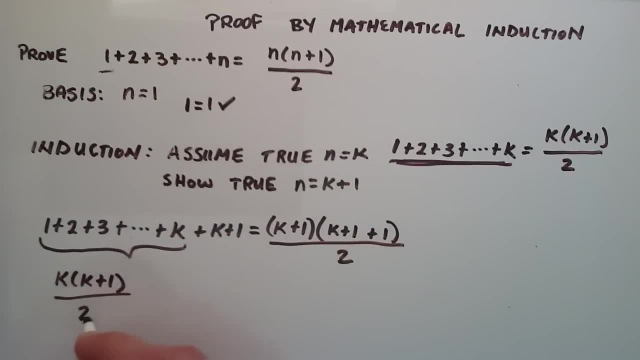 K plus one divided by two, and then we add that to the k plus one over here, And then we're just going to check: is that equal to k plus one? and then here this is really k plus one plus one or k plus two divided by the two. And then one more thing I want to do. 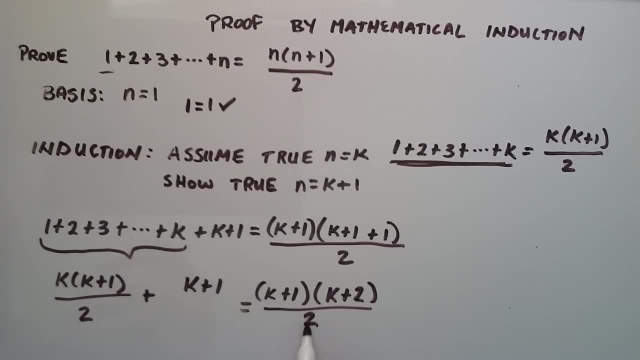 is. notice how this is divided by two and this is divided by two. I'd like to make a two denominator of 2 as well, to match for this term. so I'm simply just going to multiply this by the number 1 and I'm going to choose 2 divided by 2 to be my number 1.. Since 2 divided by 2 is equal, 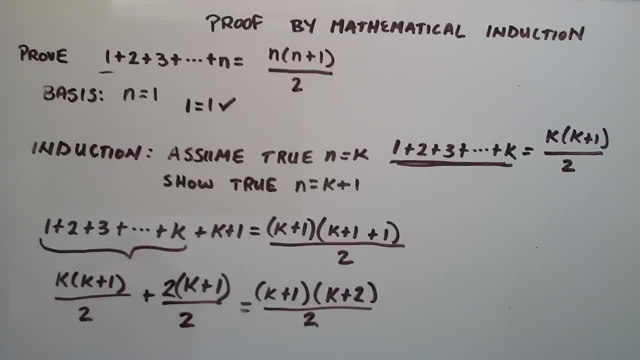 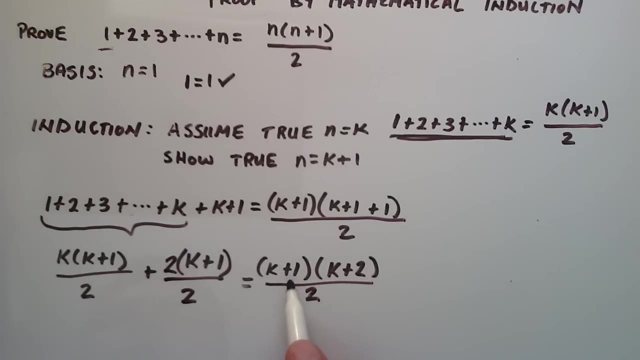 to 1. I just multiplied this by 1. anything times 1 doesn't change its value. so now I have all three of these terms with the same common denominator. So basically, if we can show that this statement is true now, then we've basically completed the mathematical induction proof. So if you notice, 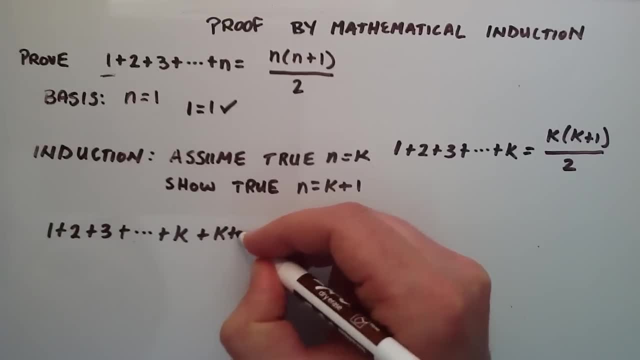 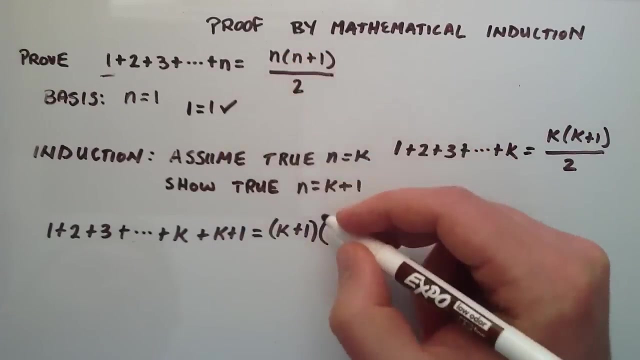 And then we go one more further to k plus 1.. And then we're going to also plug in k plus 1 where the n's are here. So this is going to be k plus 1 for that part, And that's multiplied by k plus 1.. 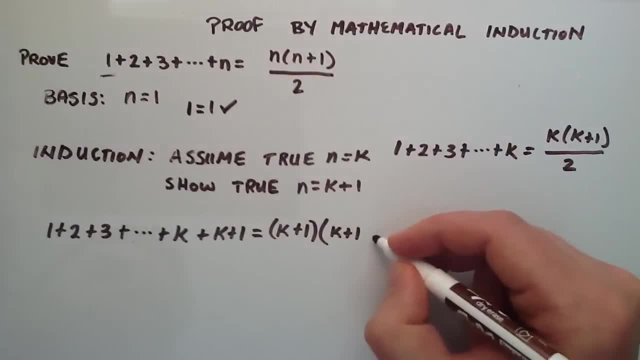 And then we have k plus 1, plugging that in where the n is, And then we have plus 1.. We could put this in parentheses to kind of set it apart, But really we're just going to be adding these anyway. 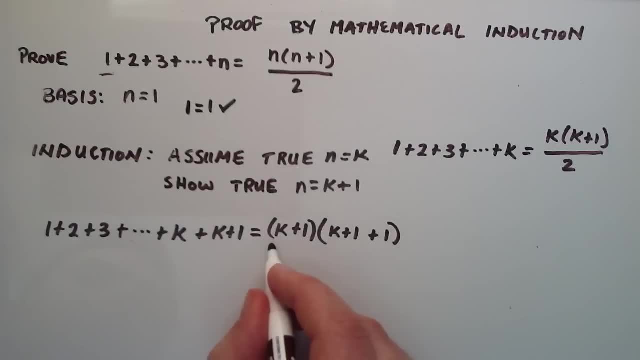 So I'm just going to leave it like this And then we're going to divide that by the 2 here. So we're assuming this is true And we're going to show that this is true based off of this assumption. So what we're going to do with this assumption is, if you notice, right here we have 1 all the way up to k. 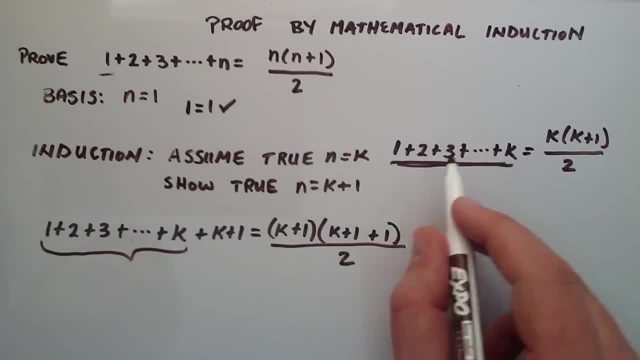 Okay, We have right here, And since we're assuming this is true, then we're basically saying that this right here we can use to replace this, because these are the same. So we're just going to replace all this stuff with the right-hand side of this assumption. 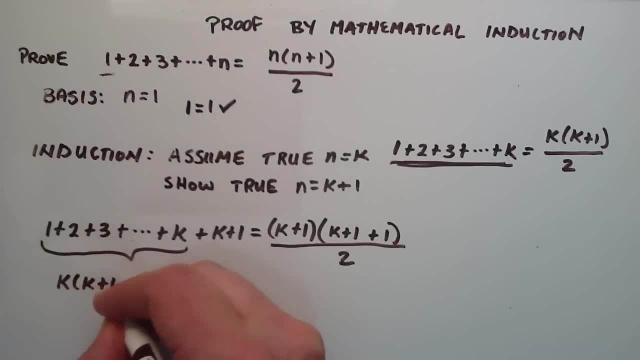 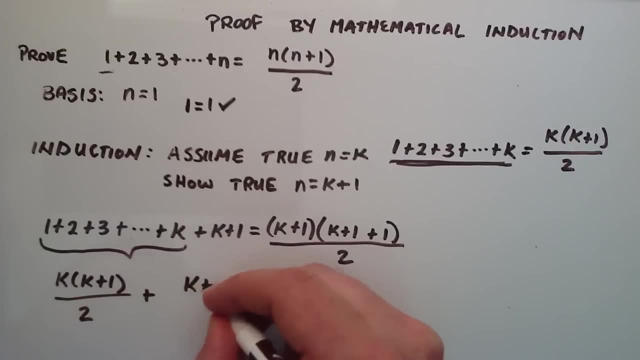 So this becomes k times k plus 1 divided by 2.. And then we add that to the k plus 1 over here. Okay, And then we're just going to check: is that equal to k plus 1?? And then here this is really k plus 1 plus 1, or k plus 2 divided by the 2.. 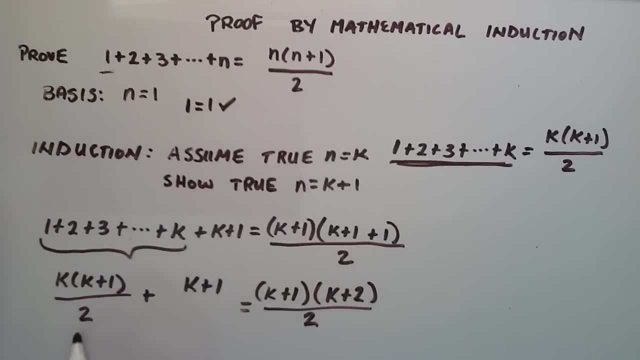 And then one more thing I want to do is notice how this is divided by 2.. This is divided by 2.. I'd like to make a denominator of 2 as well, to match for this term. So I'm simply just going to multiply this by the number 1.. 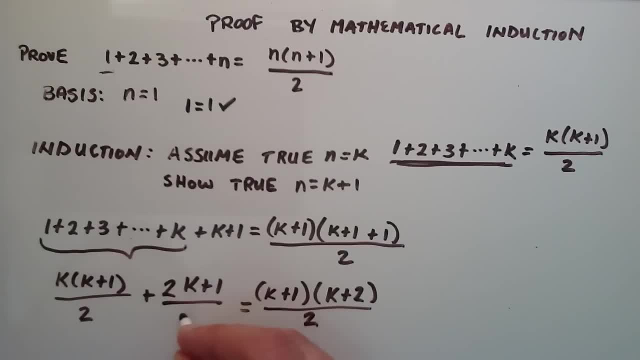 And I'm going to choose 2.. And I'm going to choose 2 divided by 2 to be my number 1.. Since 2 divided by 2 is equal to 1, I just multiplied this by 1.. Anything times 1 doesn't change its value. 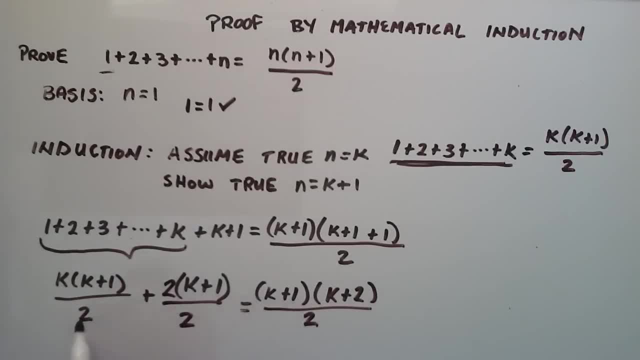 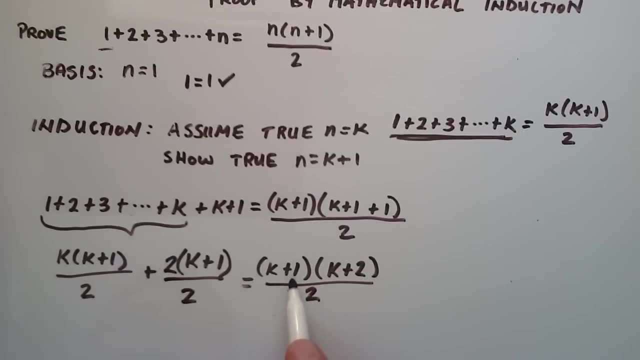 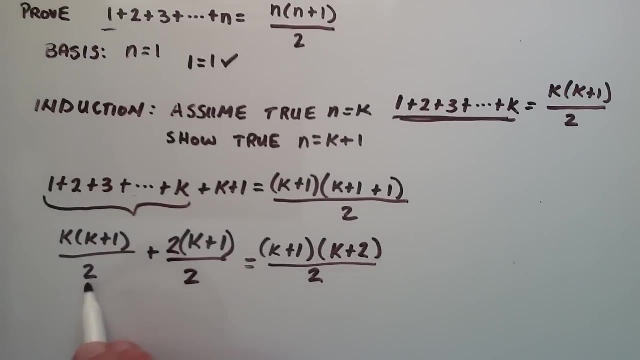 So now I have all three of these terms with the same common denominator. So basically, if we can show that this statement is true now, then we've basically completed the mathematical induction proof. So, if you notice, all of these are 2 now. 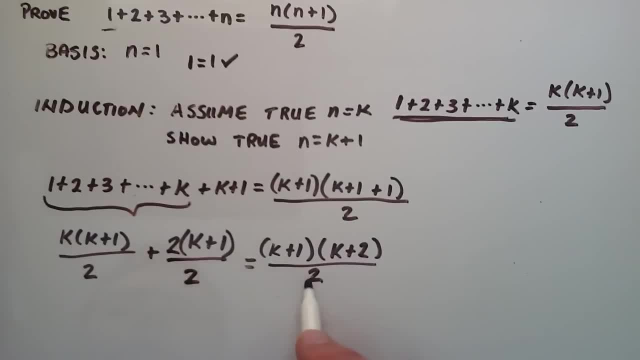 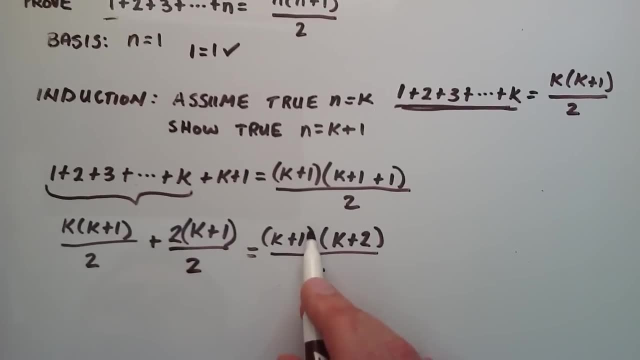 all of these are 2. now we don't even really need to look at the denominators, they're all the same. so now, if we can just show that the numerators are the same, then we've basically completed the proof. So let's just rewrite the numerators to make this a little bit more simple. k times, k plus 1. 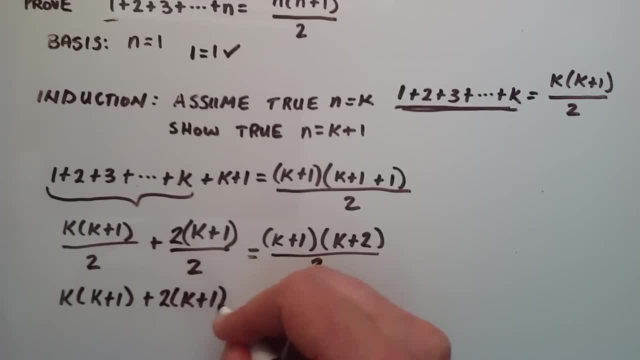 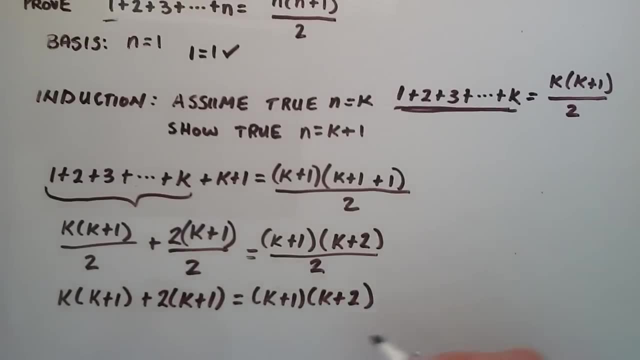 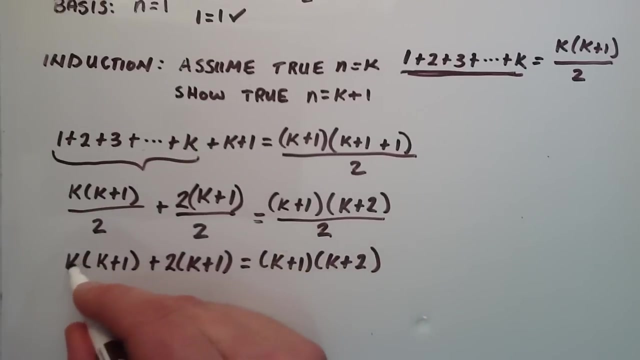 plus 2 times k plus 1 is equal to k times k plus 1 is equal to k plus 1 times k plus 2.. So now we're just going to just make sure that the numerators are the same, since we already know the denominators are the same. So k times k is k squared, and then we do. 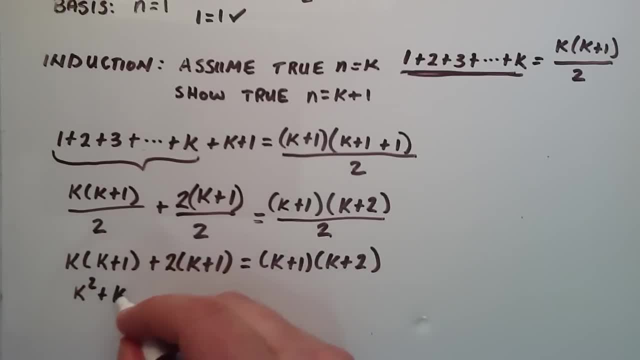 the plus distributing the k to the second term, k times 1 is k, and then we're going to add that to 2 times k and the plus distributing the 2 to the next term- 2 times 1 is 2, is that 2 times k plus 1 is k squared. So now we're just going to make sure that the numerators are. 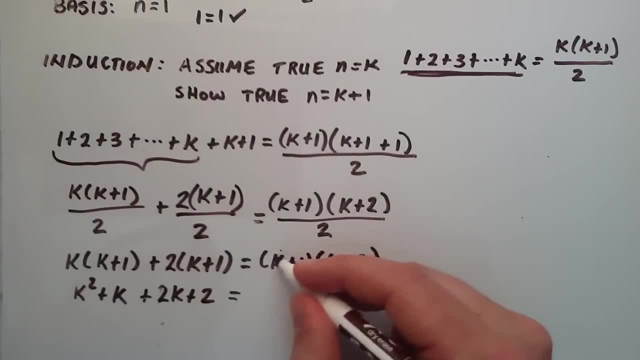 equal to기를 more than 1.. My previous control is that k div of 1 plus 1 is 4 plus 2 times 1.. t- this is going to be basically a foil. So k is k squared, and then we do the plus sign. 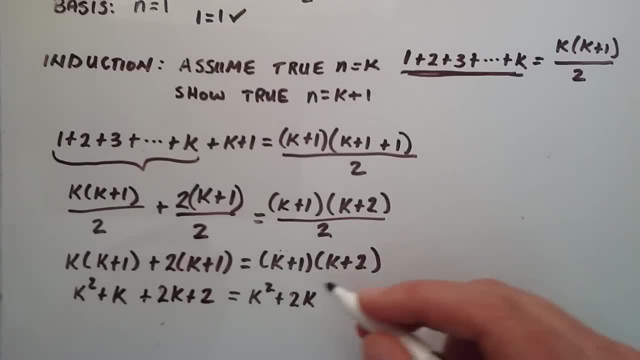 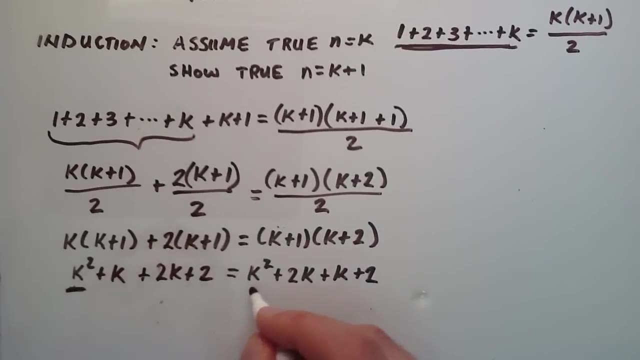 k, use the plus division to substitute the k And then for the next term, 1 times k is equal to k. k equal 1 times the positive 2 is going to be positive 2.. So now, if we look, we have a k squared on the right hand side. So now, if we look on the left hand side, we have a k squared, we have a k squared on the right hand side. on the left hand side, t is k squared. so we take that one by 2 and that's what we basically 했는데. distra 2, which is гол Network. 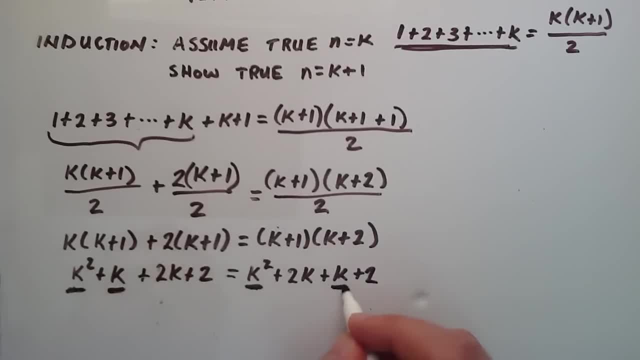 side. we have a k On the right-hand side, we have a k On the left-hand side, we have a 2k. On the right-hand side, we also have a 2k And we also have the number 2 on both the left and. 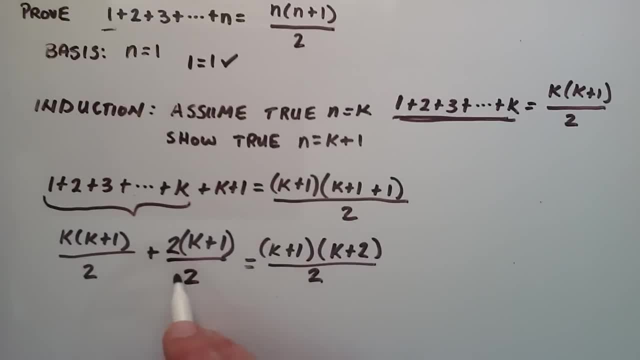 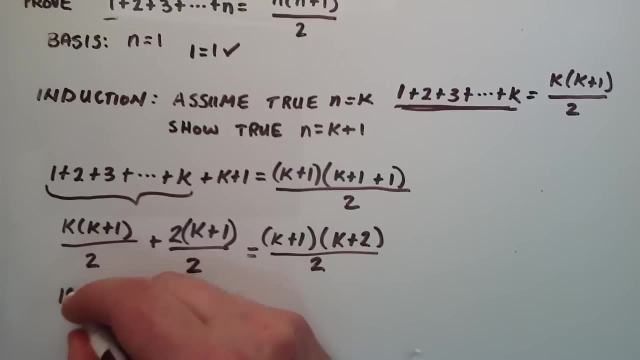 We don't even really need to look at the denominator, They're all the same. So now, if we can just show that the numerators are the same, then we've basically completed the proof. So let's just rewrite the numerators to make this a little bit more simple. 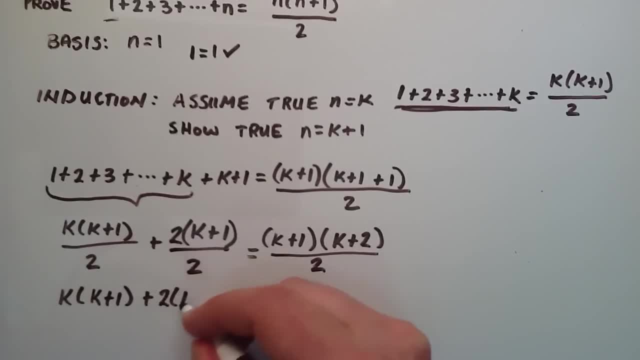 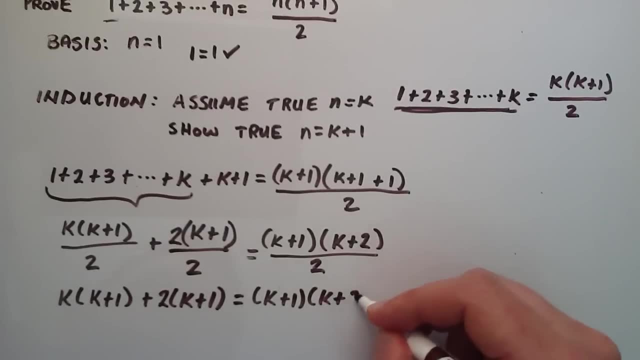 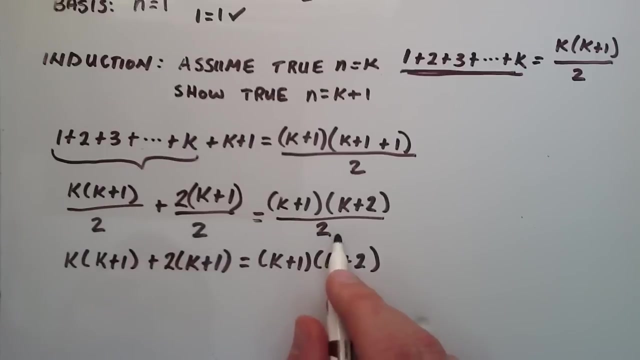 k times k plus 1 plus 2 times k plus 1 is equal to k plus 1 times k plus 2.. So now we're just going to just make sure that the numerators are the same, since we already know the denominators are the same. 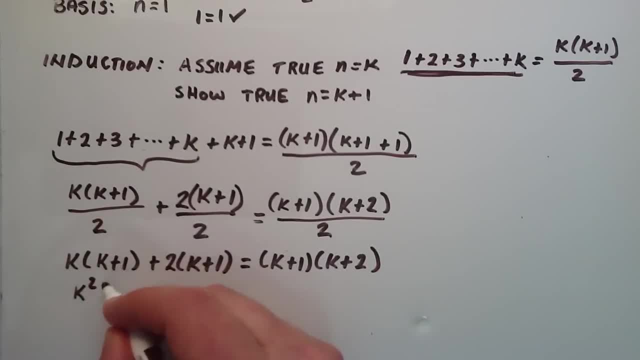 So k times k is k squared, And then we do the plus distributing the k to the second term. k times 1 is k And then we're going to add that to 2 times k And the plus distributing the 2 to the next term. 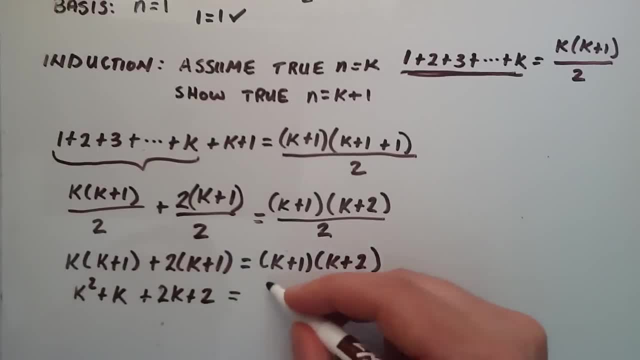 2 times 1 is 2.. Is that equal to? This is going to be basically a foil. So k distributed into the k is k squared, And then we do the plus sign: k distributed into the 2. Is 2k. 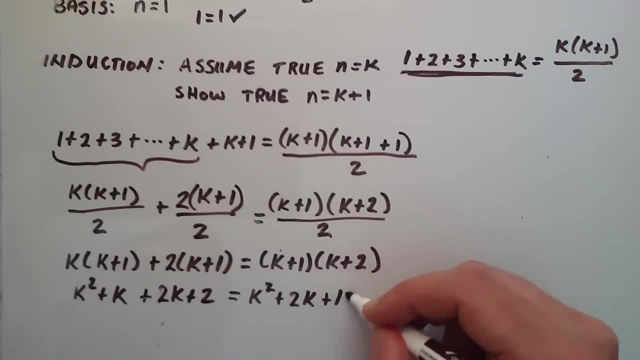 And then for the next term: 1 times k is equal to k. 1 times the positive 2 is going to be positive 2.. So now, if we look on the left-hand side, we have a k squared. We have a k squared on the right-hand side. 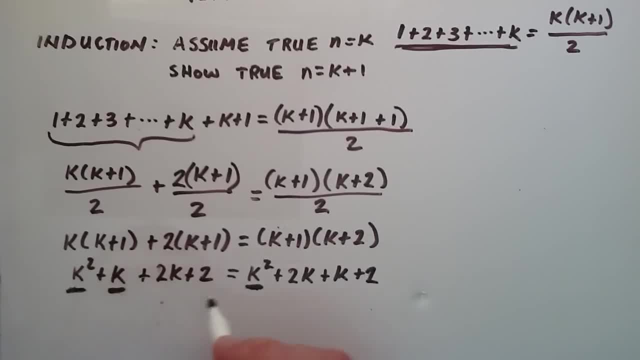 On the left-hand side, we have a k. On the right-hand side, we have a k. On the left-hand side, we have a 2k. On the right-hand side we also have a 2k And we also have the number 2.. 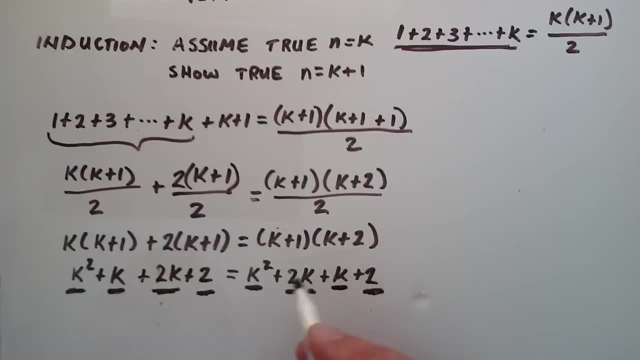 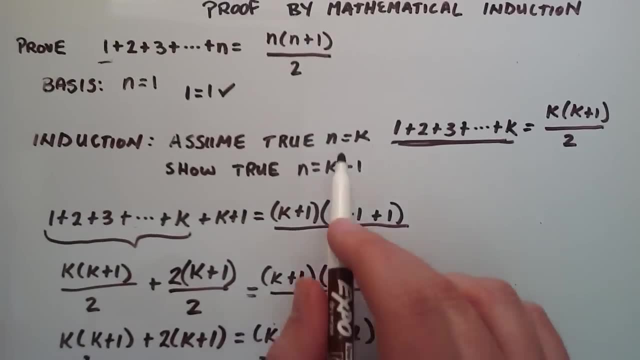 On both the left and the right-hand side. So we've basically showed that this is true for n equals k plus 1.. And we did that based off of the assumption that it is true for n equals k, And we've checked the basis step to show that it works for at least the most simple case. 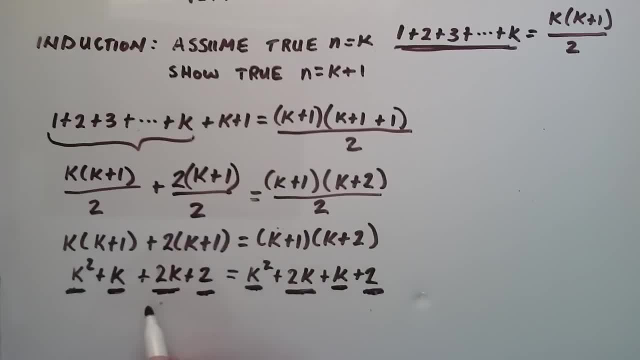 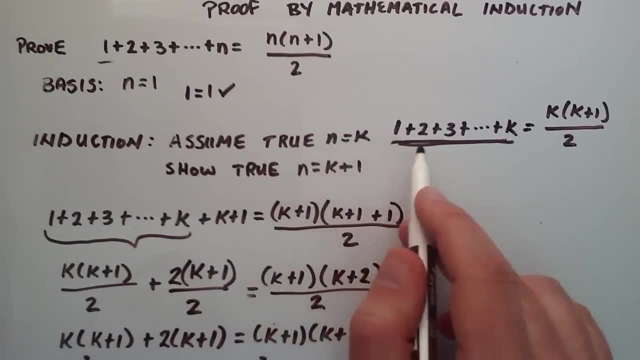 the right-hand side. So we've basically showed that this is true for n equals k plus 1.. And we did that based off of the assumption that it is true for n equals k, And we've checked the basis step to show that it works for at least the most simple case And basically that is the entire. 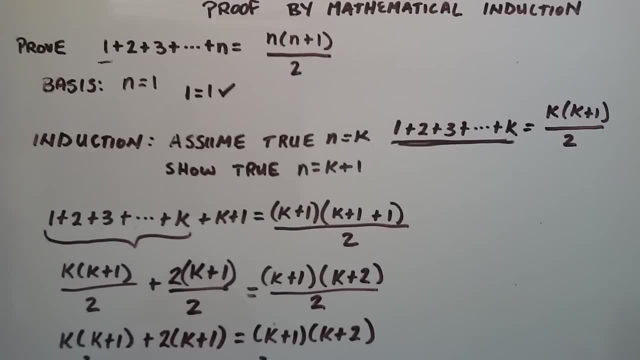 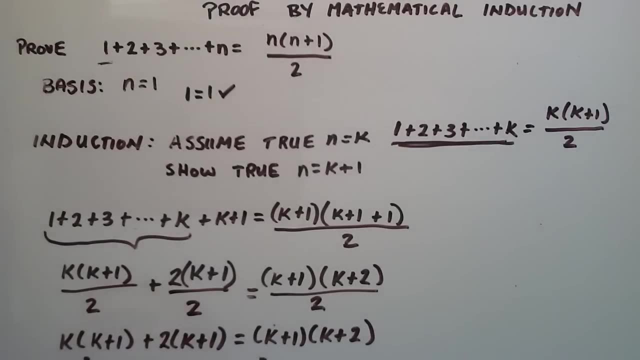 And basically that is the entire proof. right there, We have now proved that this statement is true by mathematical induction. So, anyway, thanks for watching and stay tuned for some more educational math videos from LearnMathTutorials. You guys have an excellent day. And if you haven't already, don't forget to subscribe.